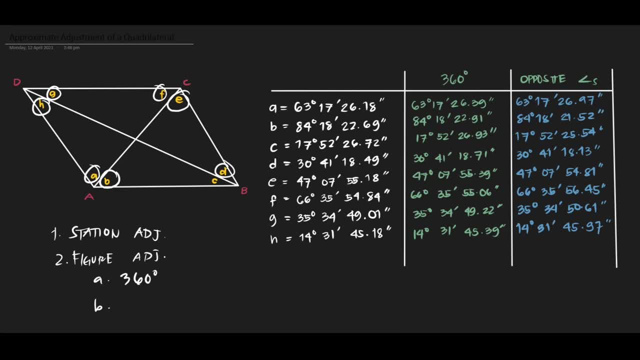 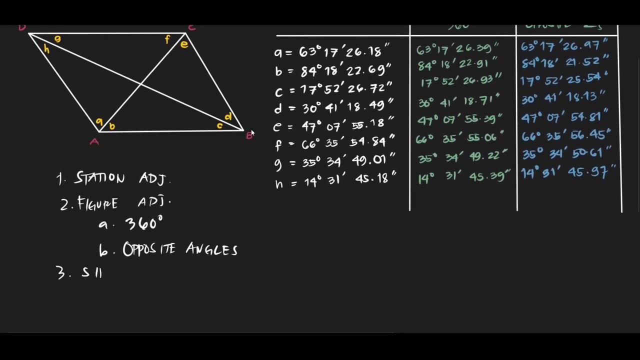 And at the same time G plus A must equal E plus D, G plus F must equal B plus C. okay, So you will see that later. So let us just write here opposite angles Now. the last one would be the side condition. 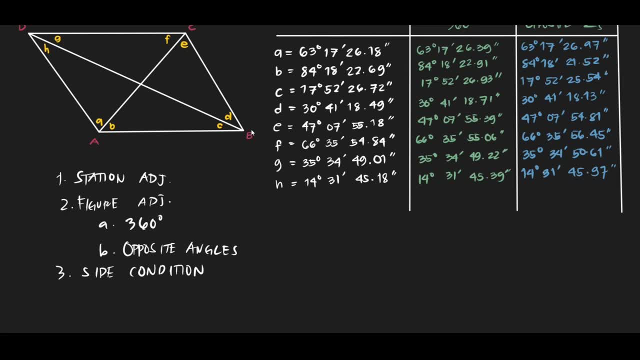 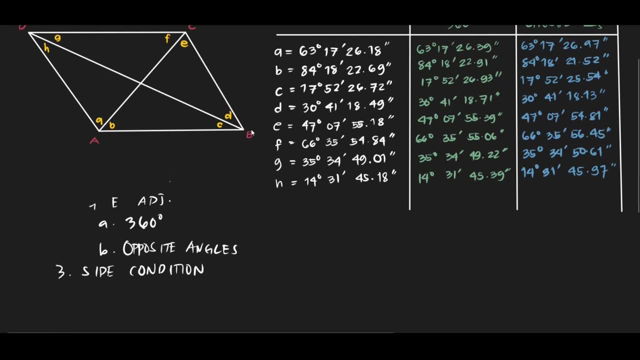 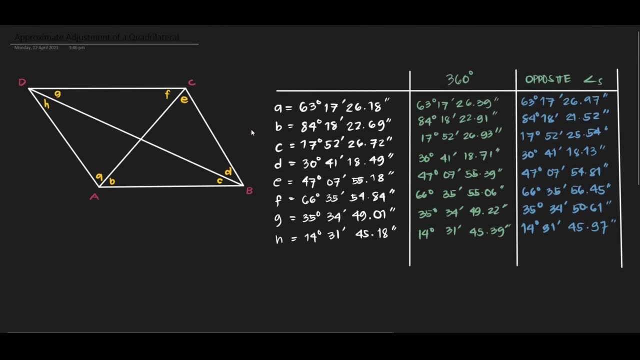 And the side condition will be discussed later. So, after we have done that, Let us now move on to the figure adjustment. Okay, so let us start. So regarding the first step, station adjustment, We can only do that if we have external angles measured right. 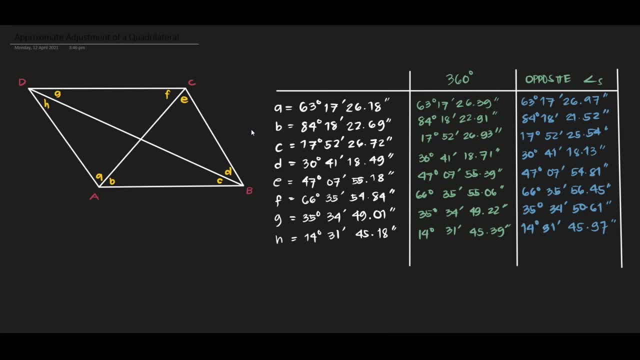 Make sure that the summation of the angles in a particular corner is 360 degrees, But for this example we do not have an external angle. A, B, C and D here are not angles, They are just the name of the corners. 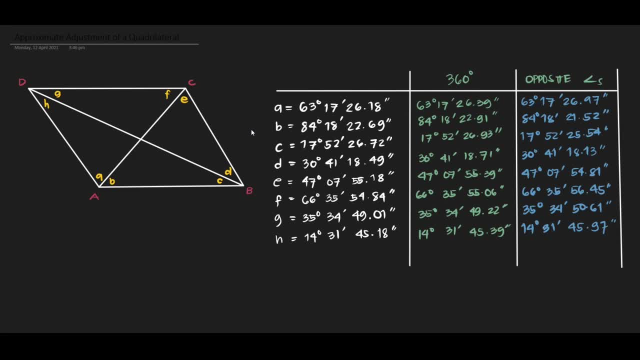 So if you do not have an external angle, then you cannot adjust for station adjustment. okay, So let us proceed right away to figure adjustment Now. as you can see here on the right, I have already written the answers for the adjustment. 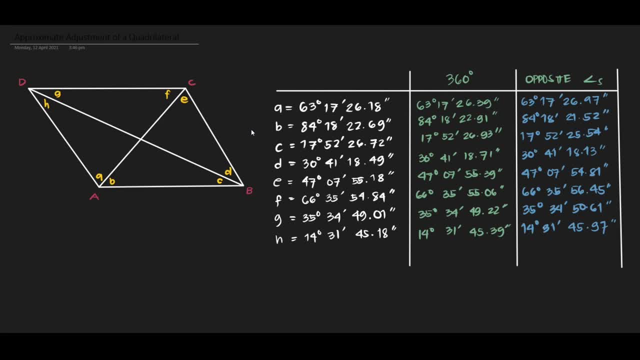 I will just explain how to do it. I will just explain how these were done. So for the first figure, adjustment making sure that all of the internal angles are, ie the sum of all internal angles is equal to 360 degrees. 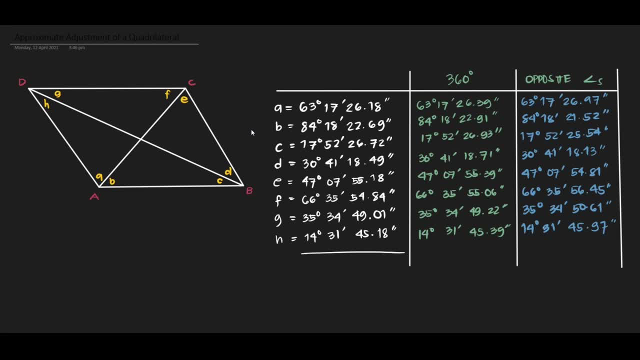 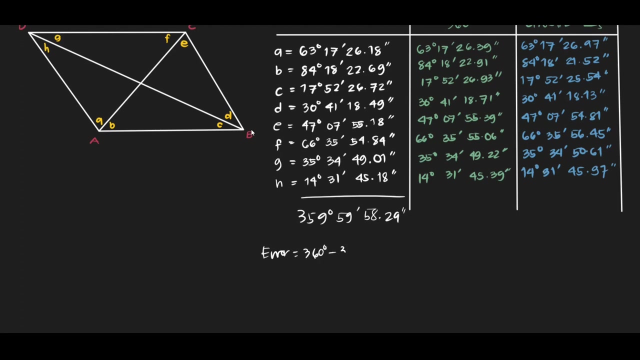 You just simply have to add all these angles. So if you add all these angles, you will get a total of 359 degrees, 59 minutes and 58.29 seconds. Okay, now, if we want to calculate the error, that will be 360 degrees minus 359 degrees, 9 minutes and 58.29 seconds. 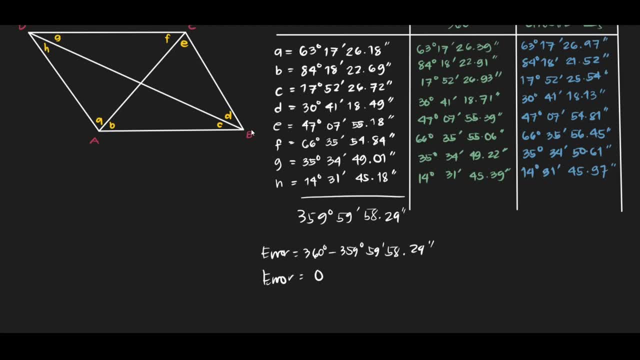 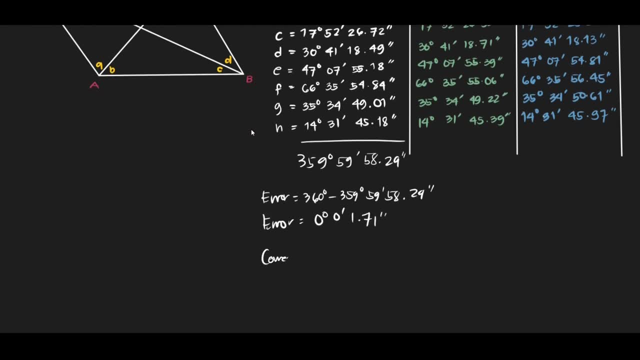 So you will get an error of 0 degrees, 0 minutes, 1.71 seconds. Now the correction will be error divided by 8, because there are 8 angles. Distribute them equally. So 0 degrees, 0 minutes, 0.21 seconds. 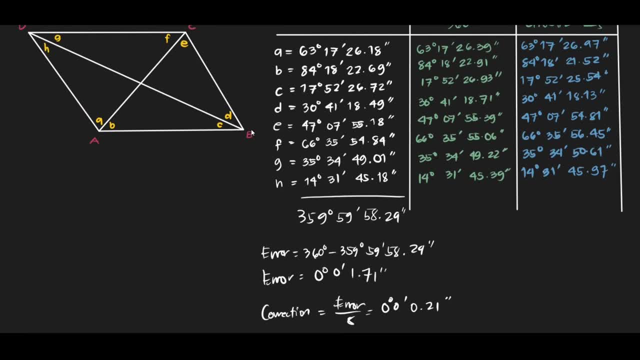 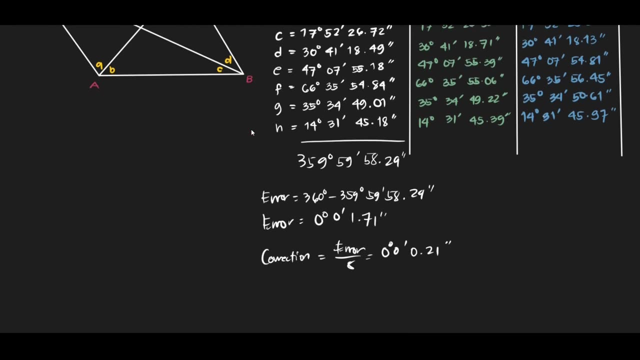 Now we need to add this to all of the angles because you can see, here the total is 359 degrees, So it lacks 0 degrees, 0 minutes, 1.71 seconds for it to be 360 degrees, So you basically have to add this 0.21 degrees to all of the angles. 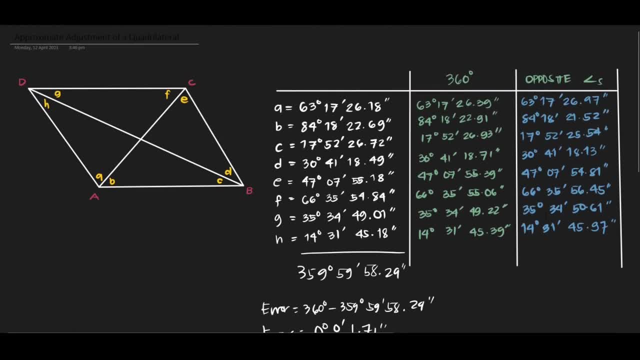 and you will get these angles in green right here. Okay, just add them to each one. Okay, so after doing that, you can then proceed to the second figure adjustment, which involves the opposite angles. So how do we do that? So let's erase this first. 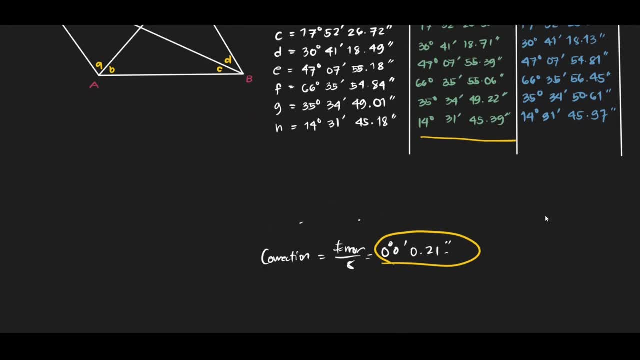 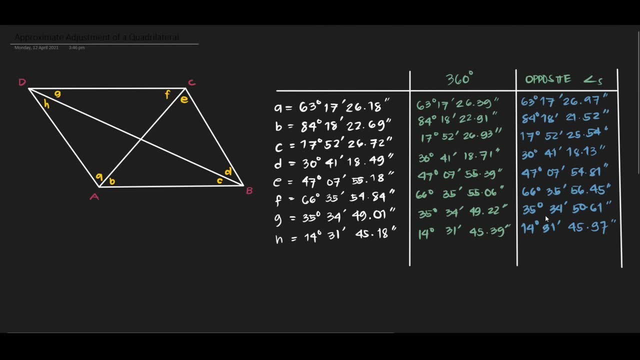 Okay. so how do we do this? So, if you take a look at our figure, we have right here, as I said earlier, H plus A must equal E plus D, right? So if we add this together, if you perform these operations, 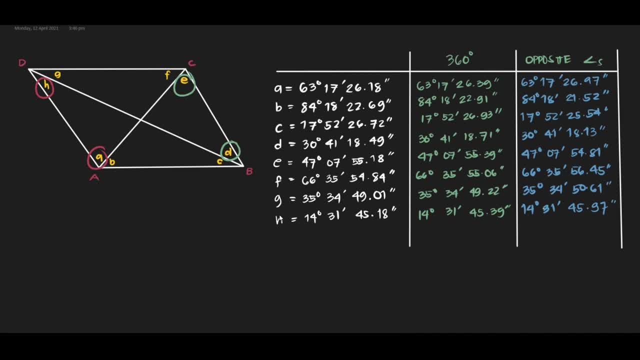 so you will get H. What is our H? So let's use the angles in green here, because these are already adjusted. So H is 14 degrees 31 minutes 45.39 seconds, plus A- 63 degrees 17 minutes 26.39 seconds. 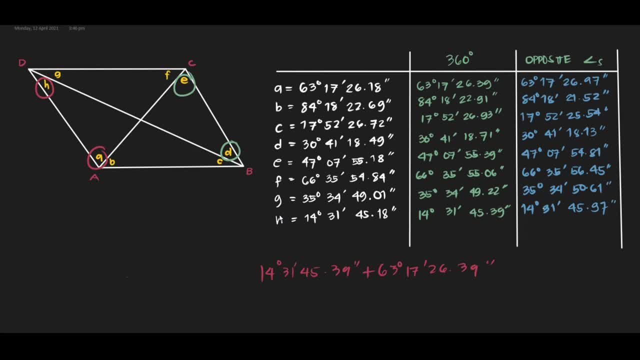 If you add that together- now let's just rewrite this, So this should be equal to E. So here is E. We have 47 degrees 07 minutes 5.39 seconds, plus D, which is 30 degrees 41 minutes 18.71 seconds. 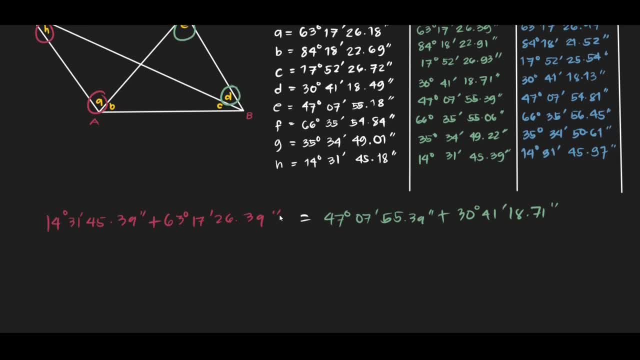 Okay, so if we add those you will get here you will get 77 degrees, 49 minutes, 11.78 seconds, And on the other side you will get 77 degrees, 49 minutes and 14.1 seconds, if I'm not mistaken. 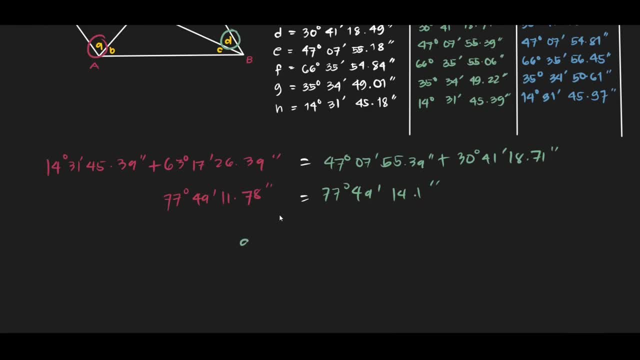 And the difference between these two. so the difference. so, as you can see here, they have obviously they have a different side. so let's quantify this difference, Let's subtract both of the values And let's just disregard the sign for now. 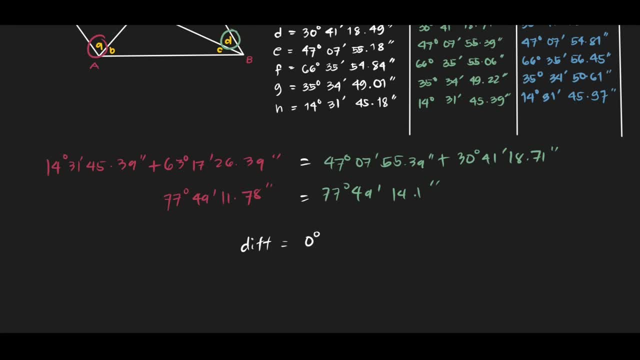 because we are concerned only with the magnitude. So, 0 degrees, 0 minutes, 2.32 seconds. Now. so for the correction. so for the correction, we divide this angle, this difference, by 4.. Okay, We divide them equally. 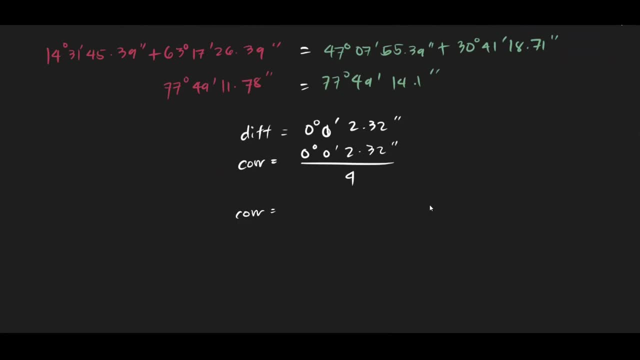 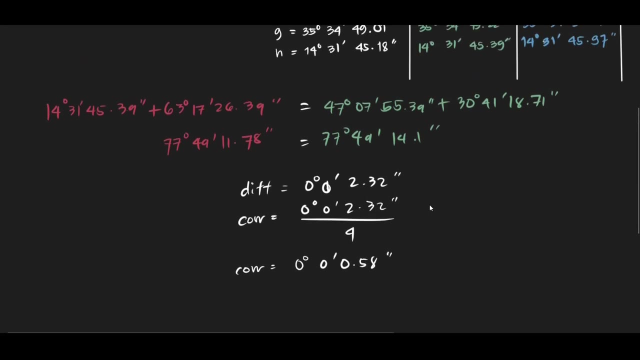 So what will be our correction? The correction will be 0 degrees, 0 minutes, 0.58 seconds. Okay, So how are we going to apply this? How are we going to apply this correction? So we must take a look. 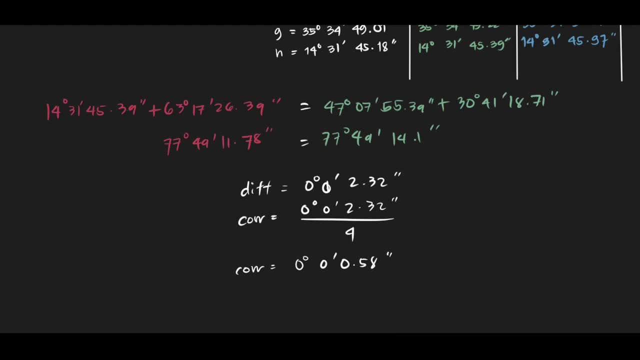 at the left-hand side and the right-hand side of our equation right here. So 77 degrees 49 minutes 11.78, and 77 degrees 49 minutes and 14.1 seconds. So the right-hand side here is greater right.